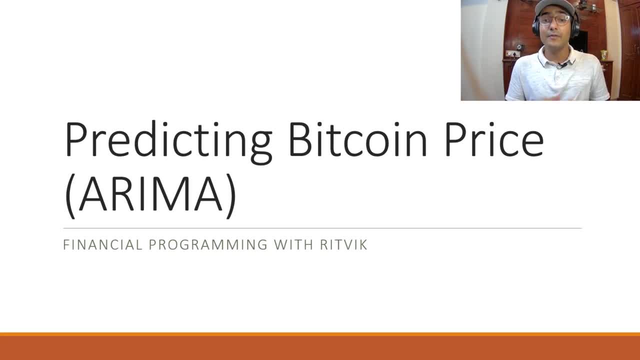 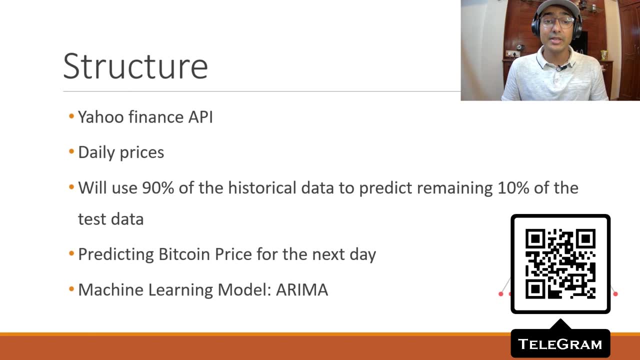 this python code. let's get started. let's understand what are we going to cover today through this ppt slides and in this video. the structure will be that i'll be using yahoo finance api, which is a free api, to get the prices. we will be getting crypto prices, which is bitcoin daily prices. in this video, i'll use 90 of the historical 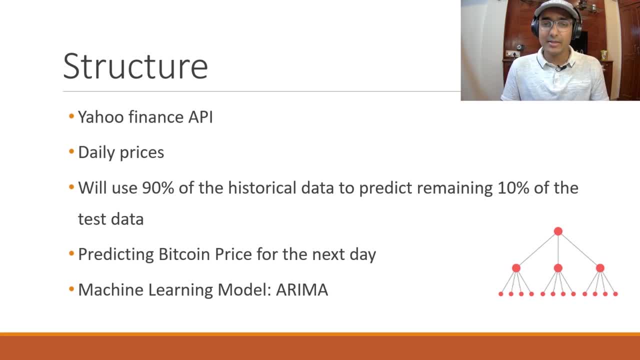 data to predict the remaining 10 of the test data. so the 90 of the data will be treated as train set and the remaining 10 percent will be treated as the testing data. right, we'll be predicting bitcoin prices for the next day, right? uh, and lastly, we are using the machine learning model, which is arima. what is arima? 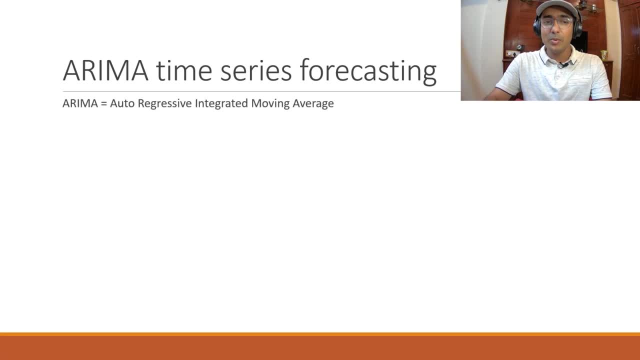 we'll cover in the next slide. so let's talk about what is. arima stands for auto regressive, integrated moving average. uh, and in this video i'm not going to uh explain each and everything in statistical point of view- uh, this video is made specifically to use a. 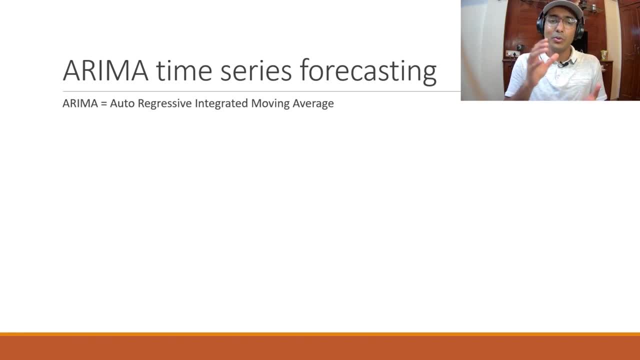 to do some time series forecasting in order to know the theoretical concepts, or maybe, like in future, i'll cover it. please mention in the comment box if you are interested to know theoretical concepts as well, or related to arima. so yeah, as i mentioned, it is auto regressive integrated. 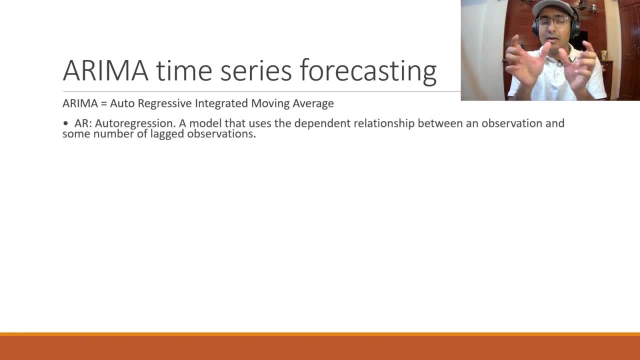 moving average. ar in arima stands for auto regression. it means that a model that uses the dependent relationship between an observation and some number of lagged observation. so in order to predict something, we are going to use some historical numbers. that is known as auto regression. integrated means that the use of differencing of raw materials, for example, 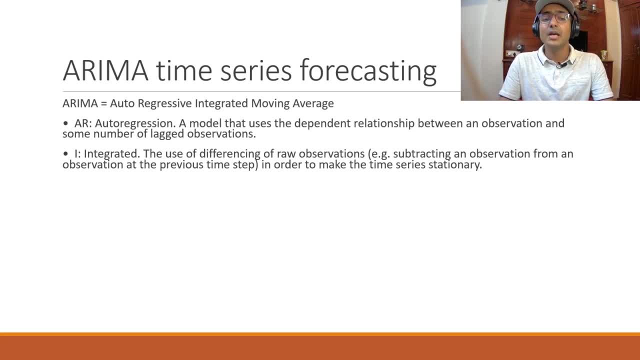 subtracting an observation from an observation at a previous time step in order to make this time series stationary. so it means that we will subtract some some of like the previous value with the current value in order to make it stationary, because there's a very high possibility. 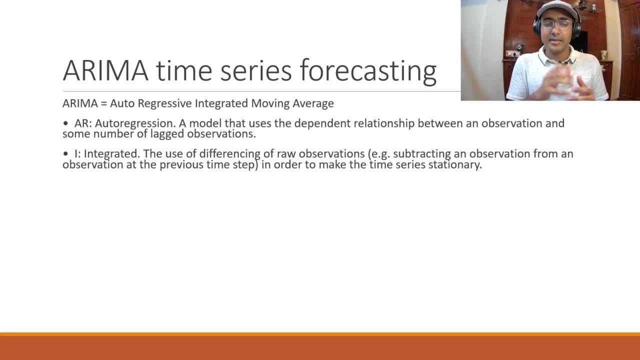 that there are some seasonal uh characteristic of that particular time series. in this case, we are using bitcoin prices, but, for example, if we were predicting something like sales of our company, it is. it can be very seasonal, so in order to make it stationary, we need this integrated model as well. 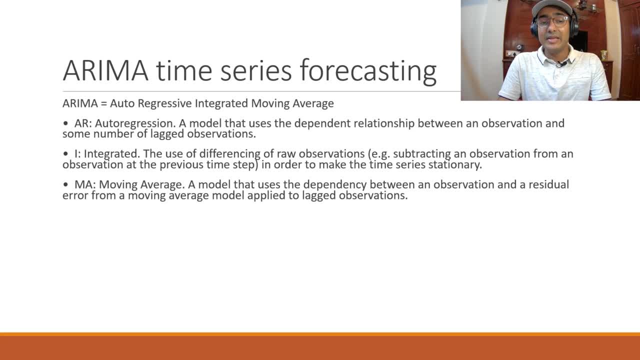 and lastly, ma in arima means moving average, a model that uses dependency between an observation and a residual error from moving average model approach to let observation. I think you would be very much familiar with the moving average. basically, we take an average of historical prices and we roll it down to 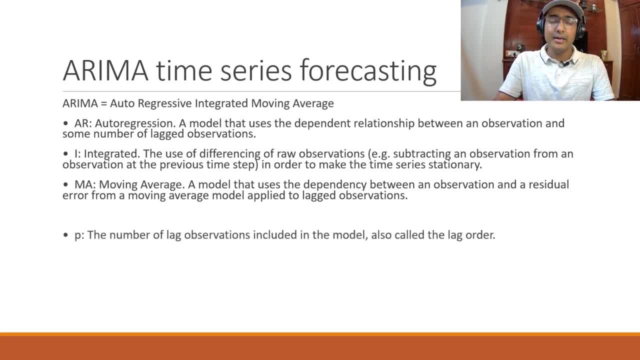 make it moving. so this is known as moving average, and there are there will be some parameters that will be used in this model. one of the most important parameter is P. it represents the number of lag observations included in the model, also known as lag order. so if, in the case of this one, the AR, we are 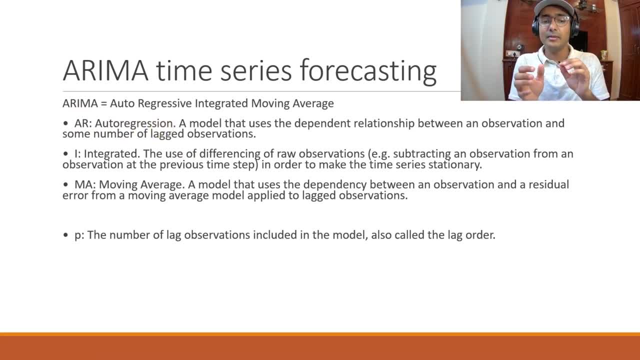 considering some lag observations. so how many the number of the lag? lag observations will be considered. that number will be used as P here, and the second one is D, which is the number of times that the raw observations are differenced, also known as the degree of differencing. so I'll come back to this. I 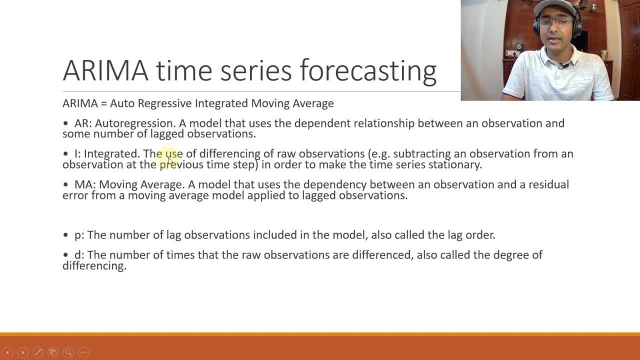 which is integrated. we we saw that we use some differencing in order to make it stationary right, so we'll have to provide a number here. what is the value of that number? to make that differences in the observation that is represented through D and lastly, Q, which is the size of the moving average window, also called as. 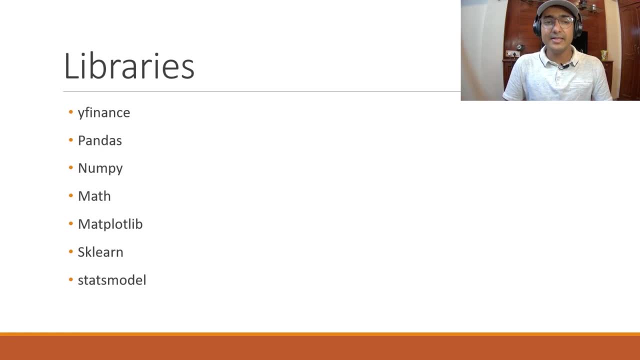 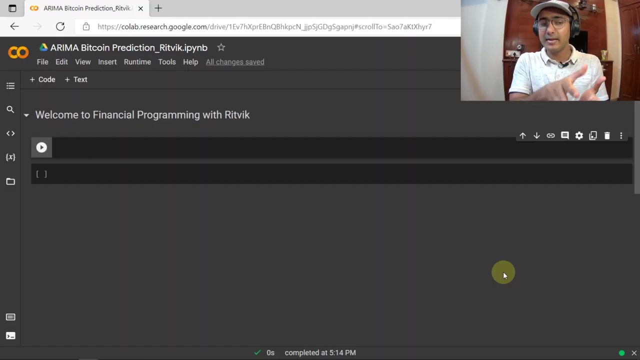 order of moving average. the libraries that we are going to use today are Wi, finance, pandas, numpy, math, matplotlib, sklearn and stats model. so, yeah, are you ready to start writing the code with me? let's start. by the way, this code that I'm going to write right now will be saved in my Google Drive and all my subscribers. 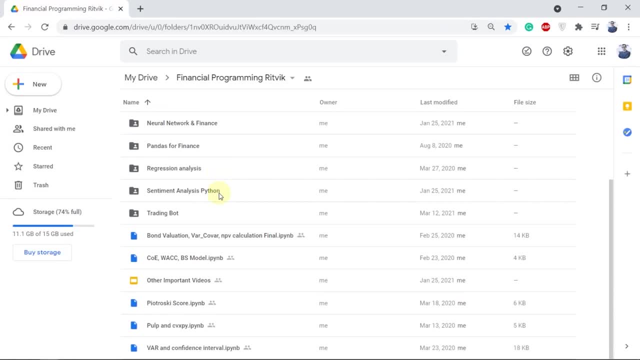 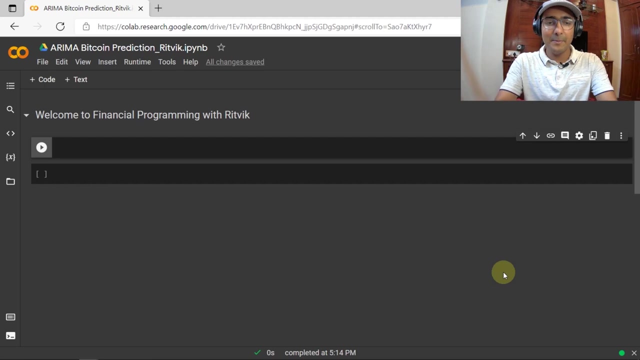 can have a free access of my Google Drive, and on that place there is a lot of things that is saved, such as my trading bot, other models, etc. how will you get a free access of my Google drive? just just wait till the end and I'll tell you how you can get a free access of my Google Drive. so let's come back to 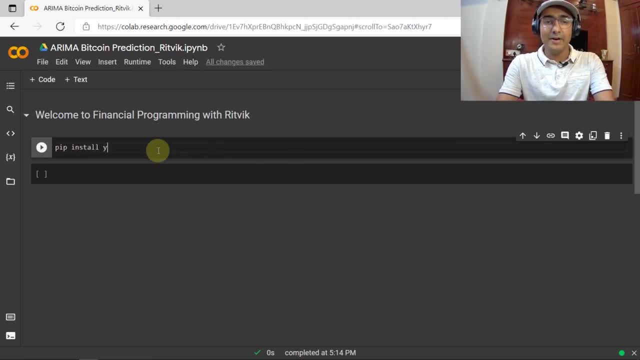 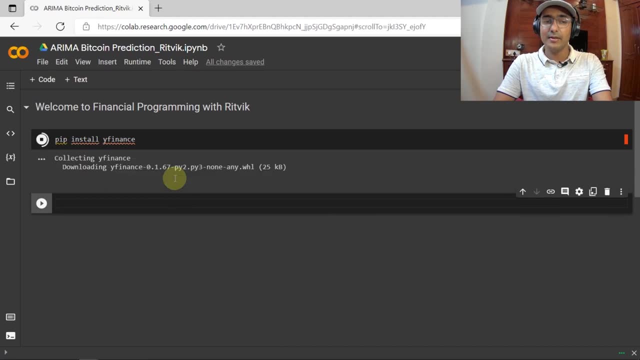 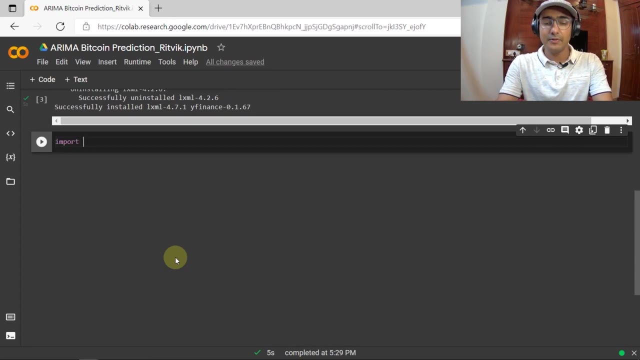 our code. I will start with installing Wi finance. there is a library that uses yahoo finance 2 all the prices required in the model. in this case, we'll be extracting Bitcoin prices using the Yahoo Finance, so let's get all the prices. first of all, import Y Finance as YF, and then DF is equal to YF, dot download and then BTC USD, if you. 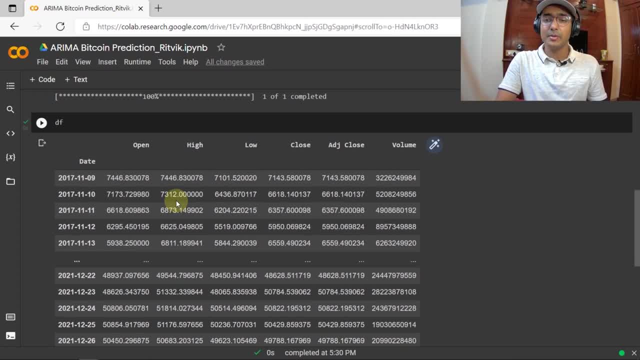 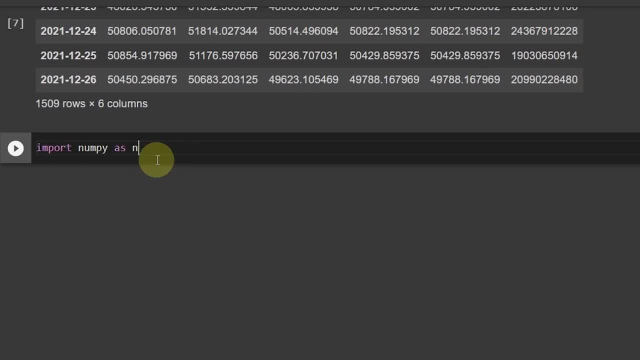 run this cell, you can see that we have got all the historical prices of Bitcoin. now let's import other important libraries: import numpy as NP, pandas as PD, matplotlib dot, piplot as PLT. let's also import math import from stats model dot, TSA, dot, arema model import arema. and lastly, which is from a skill, 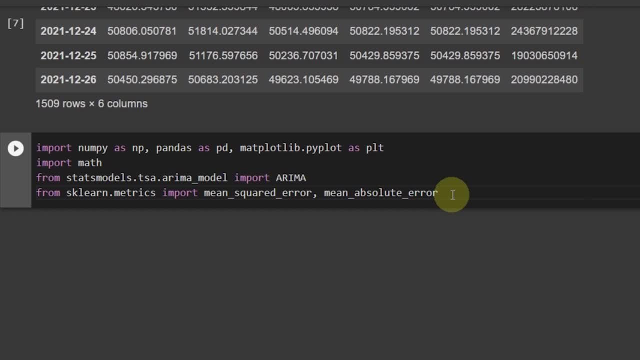 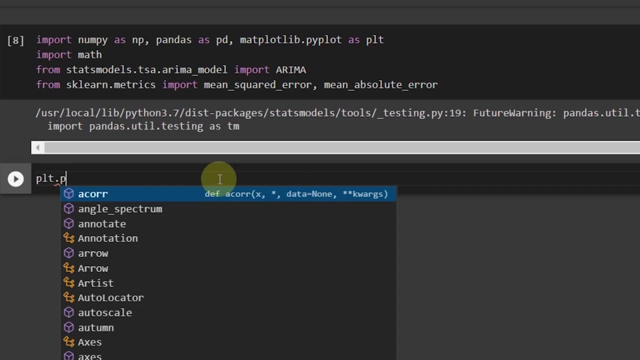 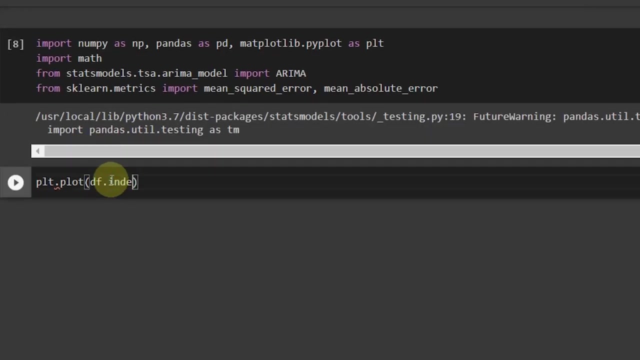 and dot matrix. import means we squared error and mean mean absolute error, perfect. first let's see the how's the chart chart chart the chart of Bitcoin prices. so PLT dot plot, DF dot- I'll have to use index here because date is in index index- and then DF at just a close PLT dot show let's see. 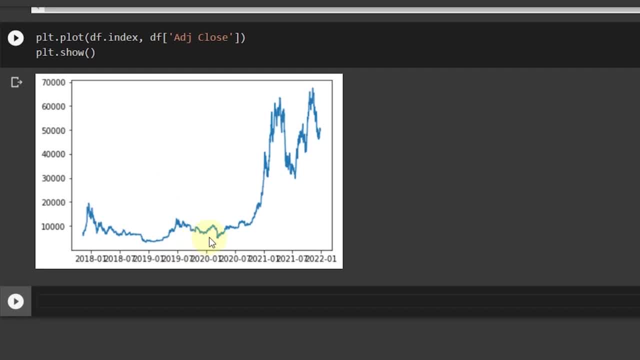 as simple as that. so you can see that how the Bitcoin prices have gone up. so what I'm going to do here is I'll use 90% of the Bitcoin prices as training set and the remaining 10% will be used as the testing set. so I'll have to. 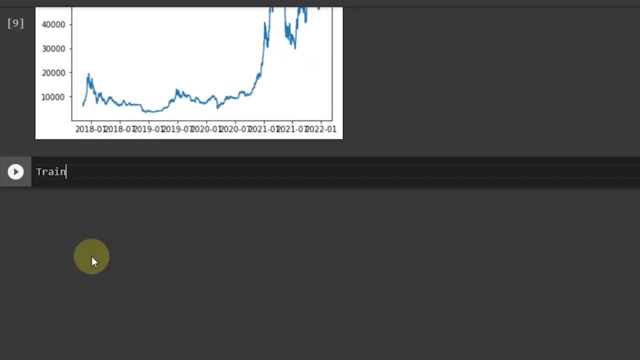 split it into two parts. let's do it train test split. so let me just write two row. I am gonna use ninety percent of the set as the testing part. so what I'm going to do here is so, if you see, len of DF, we have fifteen hundred and nine. 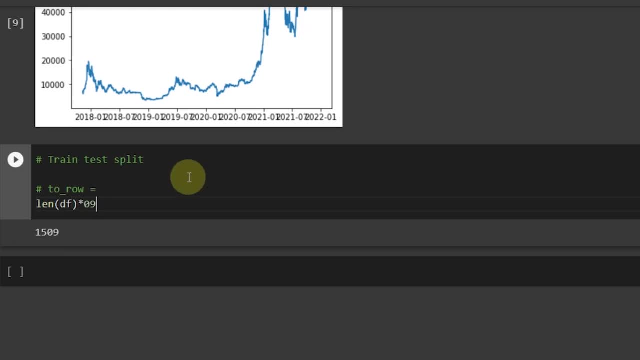 number of rows. if you multiply it with point nine, it becomes 1358.1, so I'll have to use int here. int which represents integer, so it becomes 1358. now I'm going to use this one here and delete this part. so we are using to the row which is 1358 as a part. 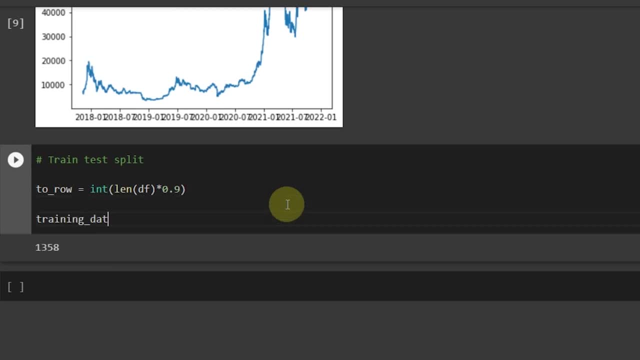 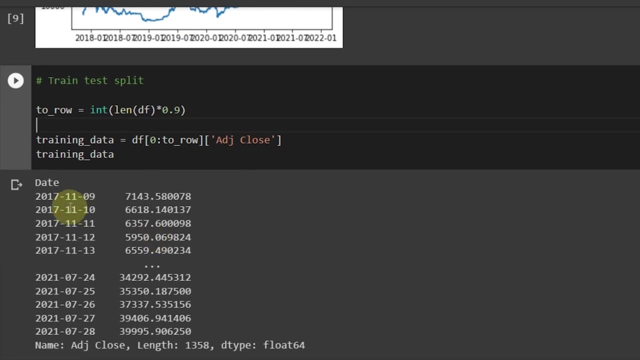 of training set and the remaining will be testing set. so training data is equal to df and then from 0 to 2 row and we are just interested in adjusted close. so if I just run this cell you can see that we have got the first 1358 rows here. now let's just convert it into list form. 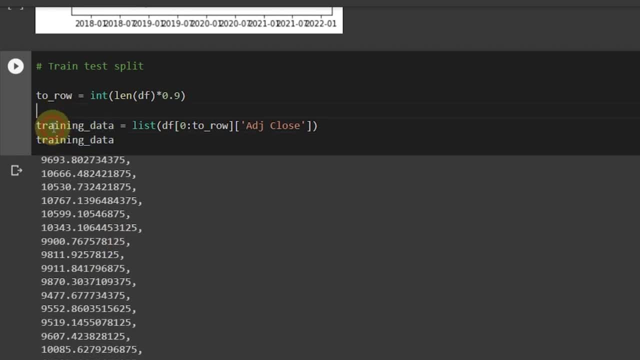 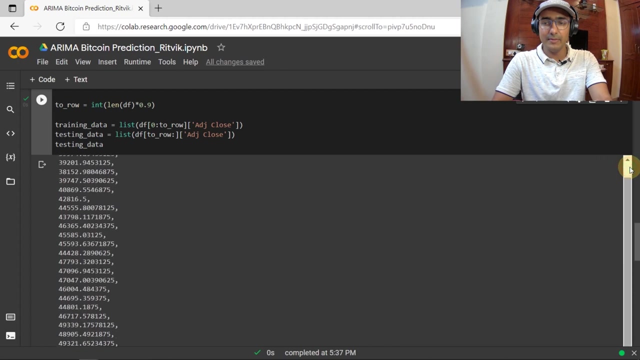 perfect, we have got the entire list of training data. let's do the same thing for testing data as well. so I'll change it to testing, and here it will be from 2 row till the end. so we have got the testing data set as well. perfect, I'll delete this part and run. 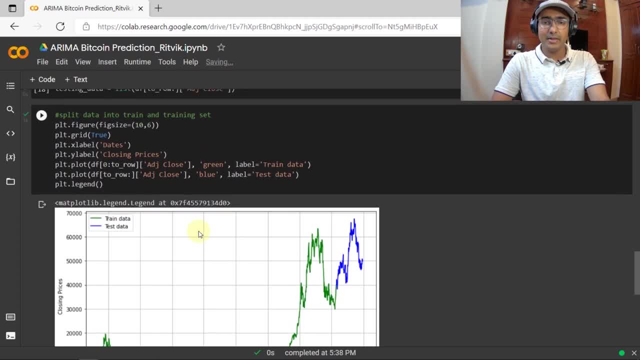 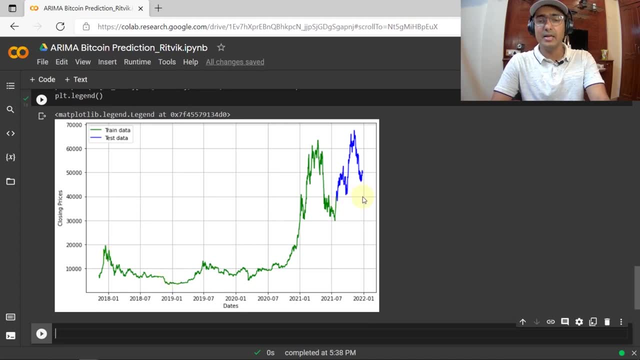 so, in order to show it again in the graphical format, as I did here, it was a bit confused, confusing here. I just split it into two parts. so this part is the green part is the training set and the blue part is the testing set. I'm just using matplotlib library to make this graph. it's 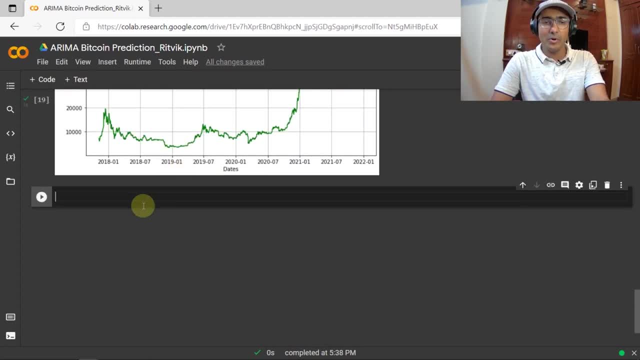 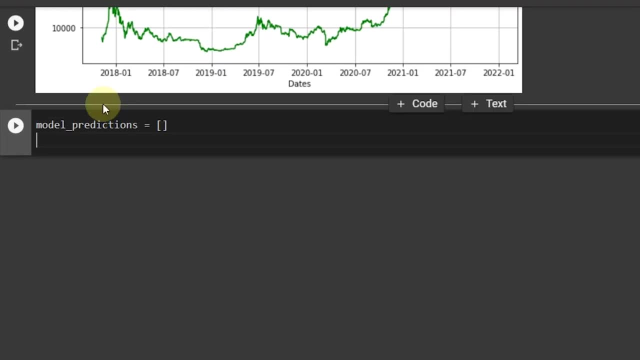 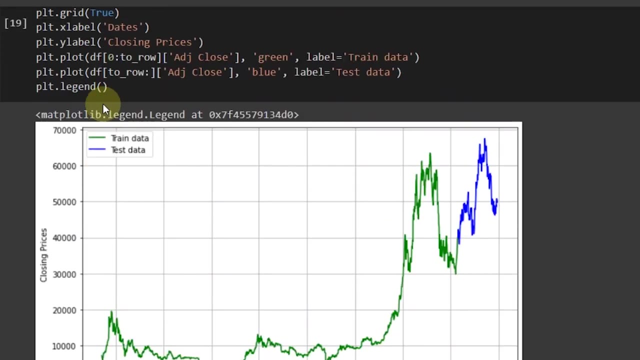 not that difficult, so I'll just quickly go to the arima model now. for that I'll have to start with model predictions as a, as an empty list, and the number of observation. the number of test observation is equal to the length of testing data. if you can see, this is the testing data and 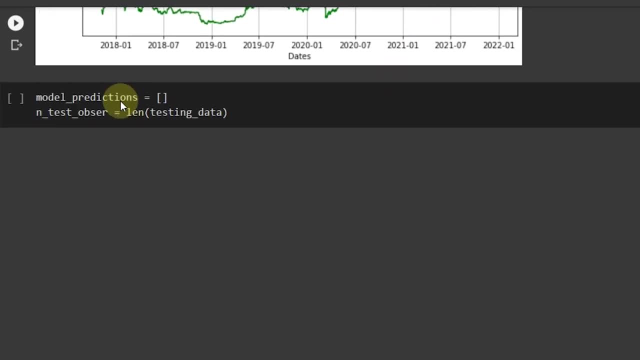 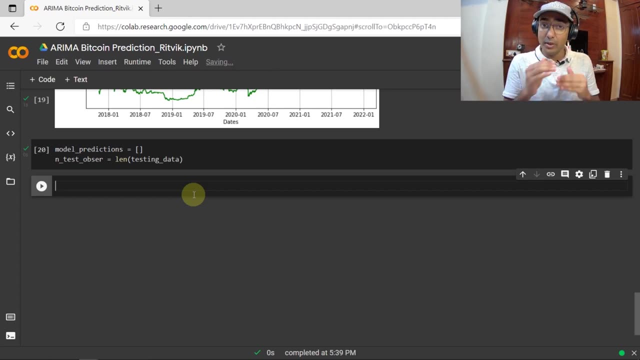 the length will be the remaining 10 percent of the entire data set. right now, what I'm going to do is I will write the arima model, which will be rolling model because we are using historical data in order to predict the future data. so if, in case of a test model, we have a test model which is 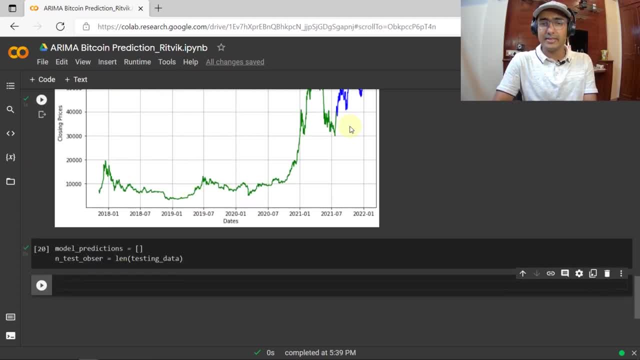 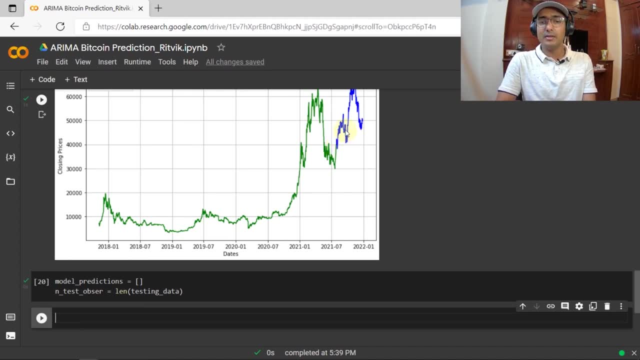 in case if it starts at t is equal to zero, for example. in this case, by saying t is equal to zero, I mean at this point, if it starts, then as we go in future, the, the window, the historical window that is considered in the arima model, should also be increasing right, so we'll have to change the 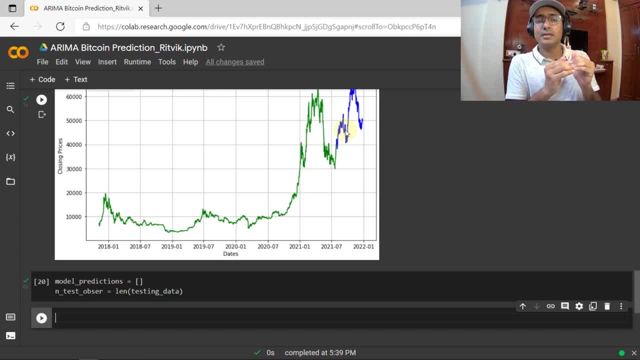 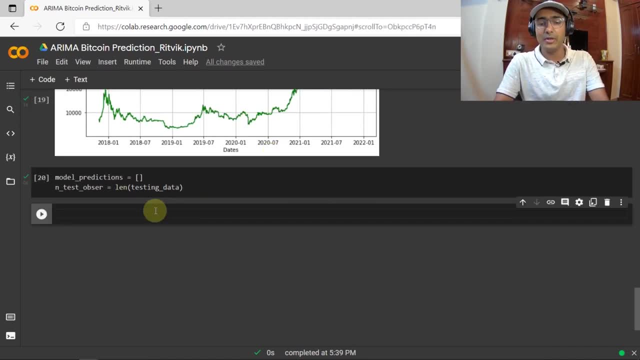 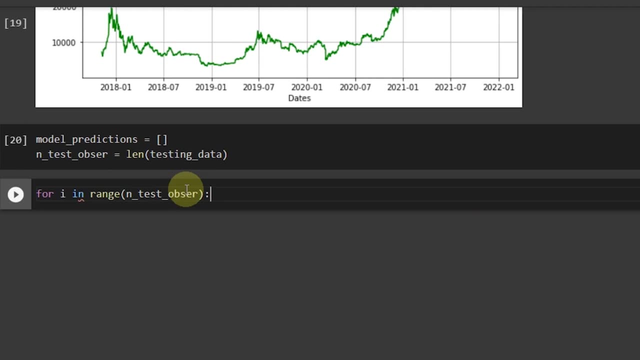 training set for all the iterations, and then that will be used to predict the prices. so for that, in order to do this thing, I'll have to just write one for loop to do this work. so for, in range of the n test observation, this is the number of observation. 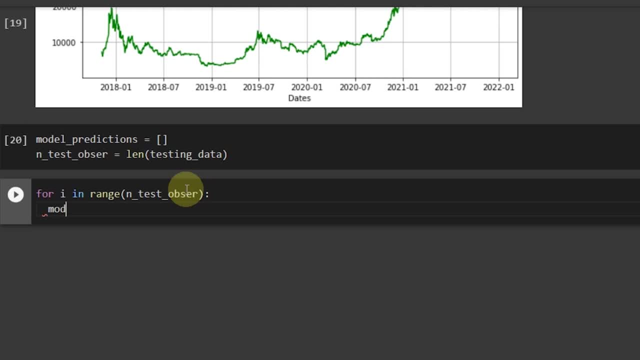 the testing data set I will write model is equal to arima. arima, and I'll be using training data as an input here. now the the most important thing, which is the order, would be equal to, let's uh say, four, one and zero. so these are the value of p, d and q, right? if you remember, I explain everything. 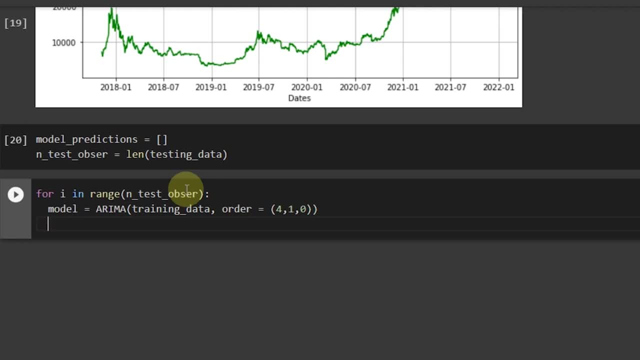 in the ppt slides. so I'm just taking four, one and zero here. you can play with different numbers to get to different type of models. now, simply, we just need to fit the model. model fit is equal to model dot fit. so that's it. let's do one thing. output is equal to. 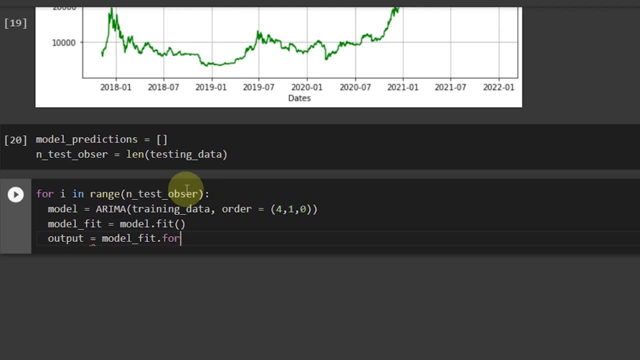 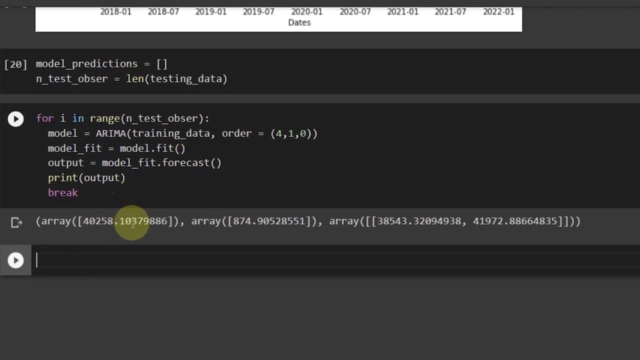 model fit dot forecast and let's print output. what is our output? I'll have to break this model, uh, this, this for loop, because it will take some time to do it for all the iterations. so you can see that the output is basically. there are different numbers here, right, and I'm just 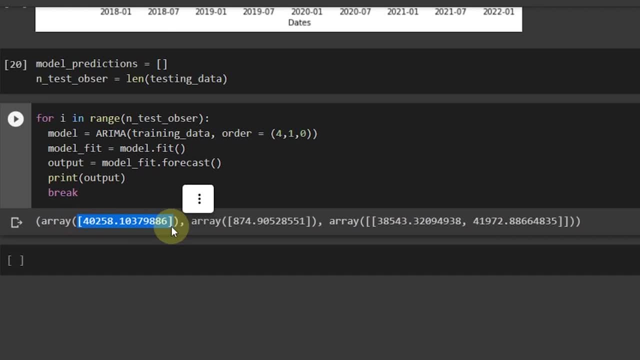 interested in the first one. this is the actual prediction, which is also known as y hat. all mathematical guys would understand what is y hat. it represents the predicted value uh of y, uh, and we will then compare it with y actual to get to know the accuracy of our model. so I'll 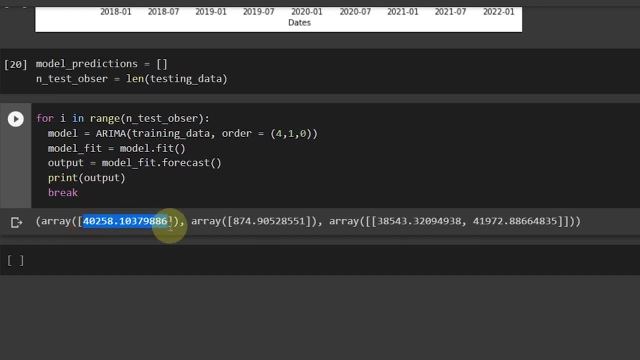 repeat, I'm just interested in this first value. so what I'm going to do here is: let me just write output here, and I'm just interested in the first one, so I'll just write zero. it's perfect. now this is in the array format. I'll have to convert into list format. so this is list, and again in this one. 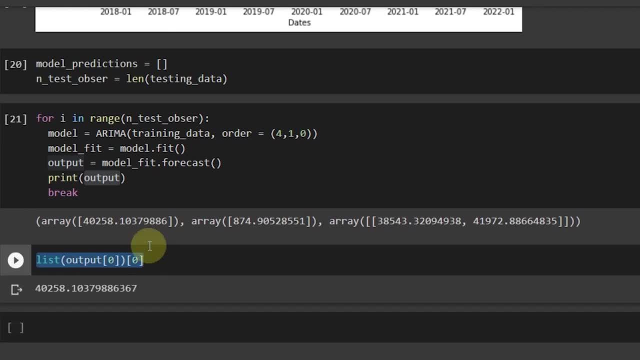 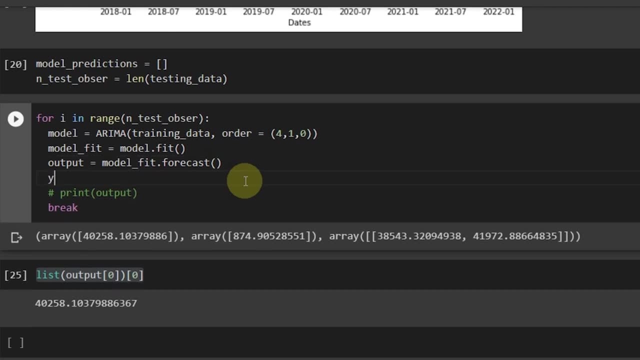 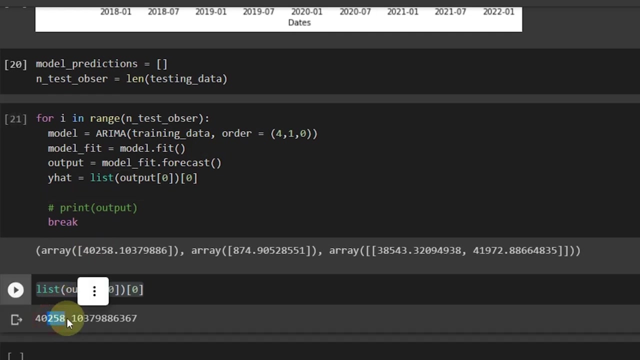 this one, so I'm interested in this number. this is the actual prediction, so in the next one I'll just comment this up: and y hat is equal to this thing, right? this 40, 258 is the first prediction, right? so what I'm going to, what I'm doing here, is I am making this model predictions list and I 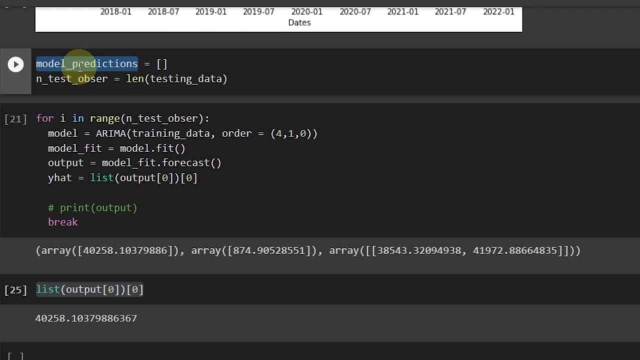 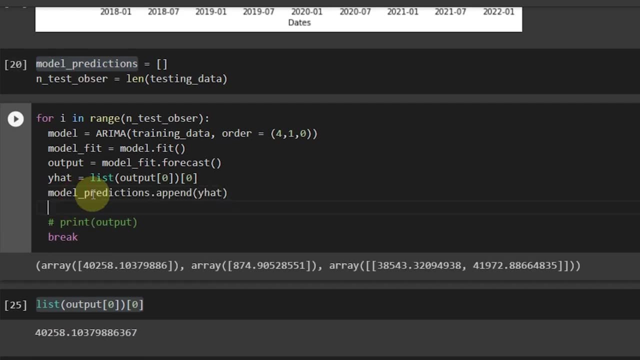 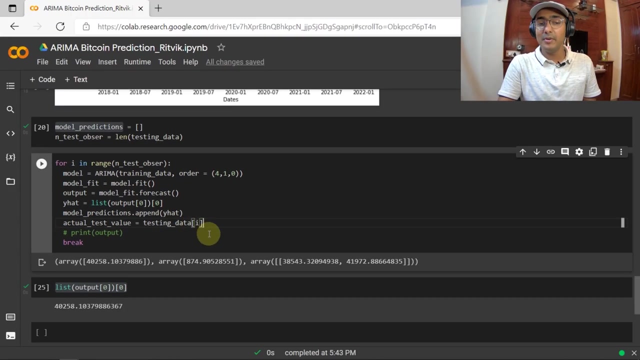 will be appending all the different predictions which will be used to plot the graph eventually. so what I'm going to do here: modelPredictionappend, and then y hat. whereas this is the value of y hat, the actual value of y, which is actual test value, is equal to testing data. and then i so, if you remember, test testing. 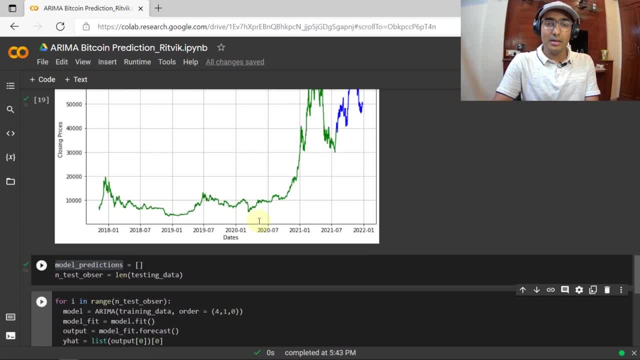 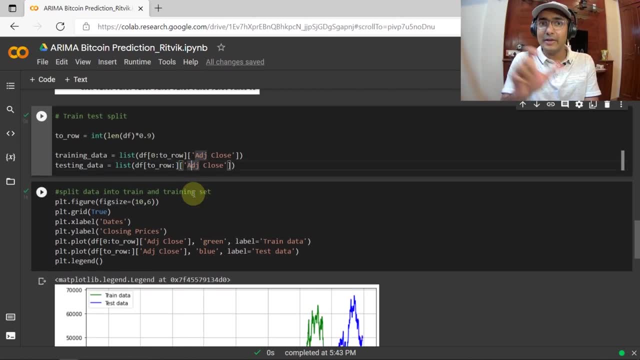 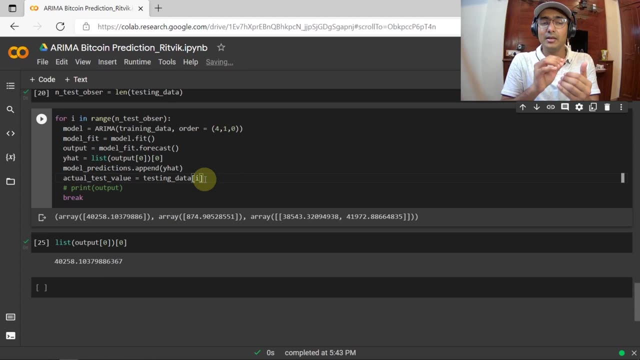 data is also a list. if we go a bit here, you can see that testing data is also a list of all the numbers, all the actual adjusted close values of bitcoin, and we we have this list, and by by writing i i mean for different iterations- we are getting the actual value, so the actual test value is equal. 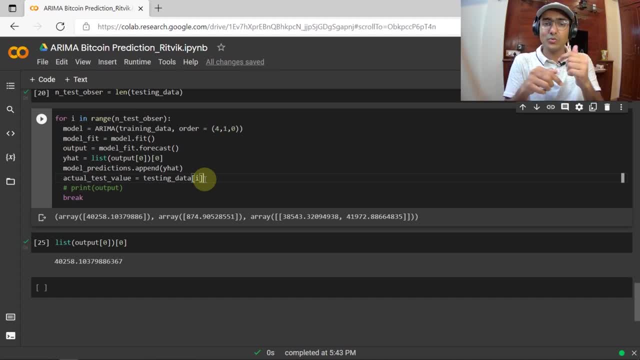 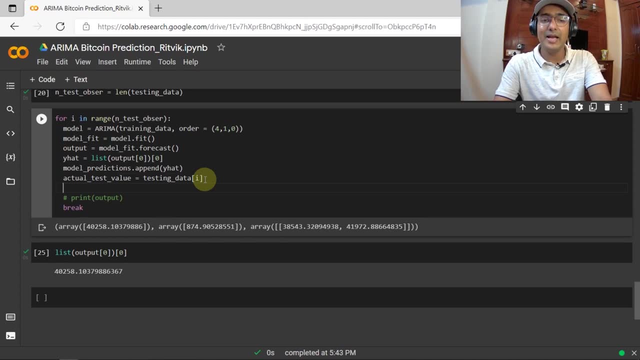 to testing value and then square brackets i. in the first one it will be square brackets zero, so it will take the first value in the list. so now what i'm going to do here is i will have to update, keep on updating the, the training set, because this training data is will be used again in the arima model for in the second iteration. 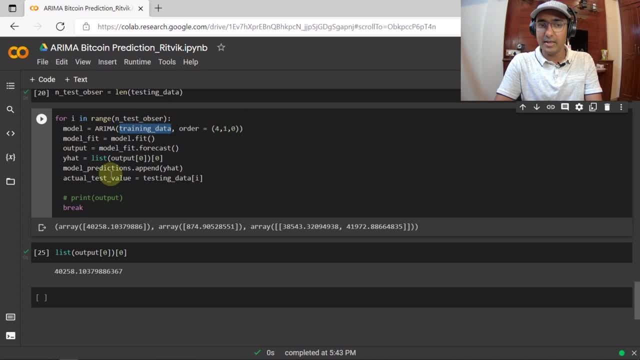 and this training data should be updated with the new value right. why? because all our models, all our future models, should be updated with the new training data. because our predictions is on the basis of the historical data and in order to reflect all the historical data, we need to keep. 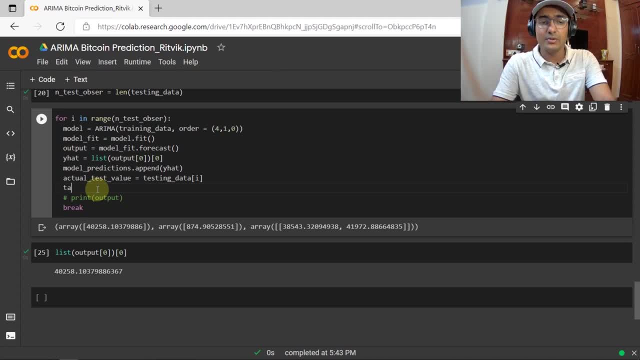 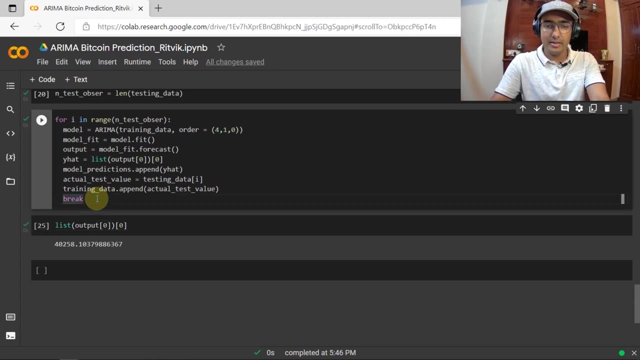 on updating the training data set as well. so training data data dot. append- actual test value. that's it. so let me keep this break for now and run it, so there's no error here. i'll. i can comment this break or let me just delete it entirely after. 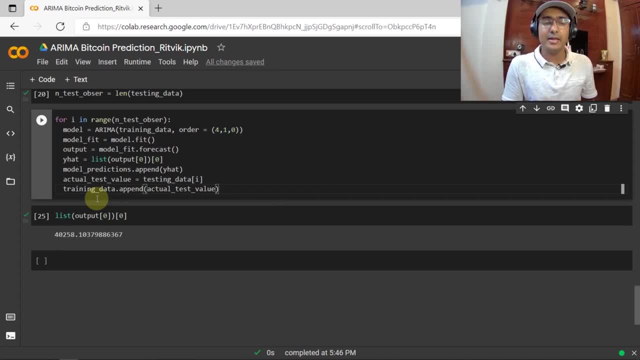 running this cell. it will take some time, so i'll have to pause this video for a moment and then we'll see what is the final result. perfect, so we have run the entire model. now let's do one thing. model fit dot. summary. let's see what is the final result. so we have run the entire model. now let's do. 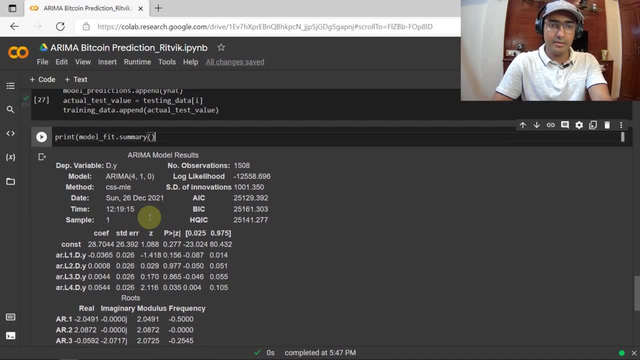 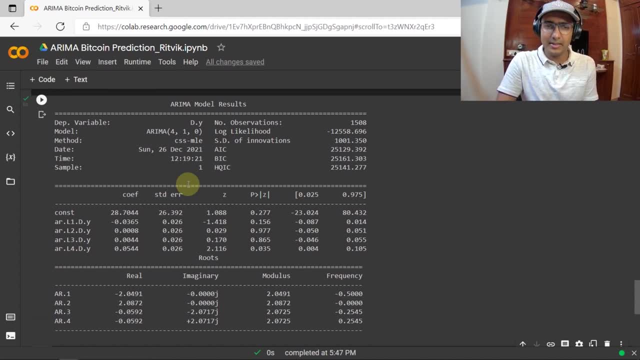 the final summary, let me just write print here: perfect. so this is. these are some of the numbers that will give you an in-depth analysis of the entire arima model to you. you can see that the model that we ran is 4 comma 1 comma 0, which are representing the p, d and q variables respectively. 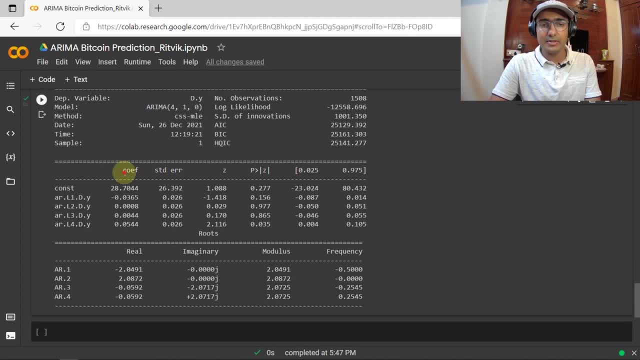 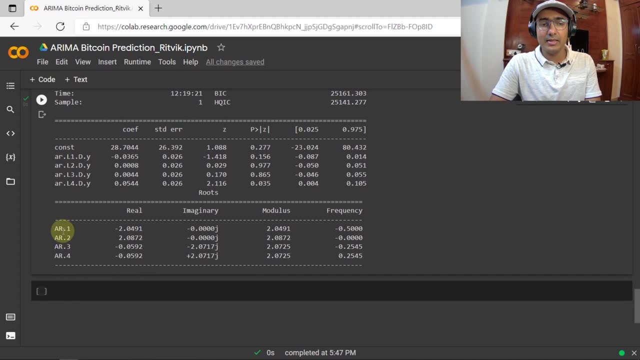 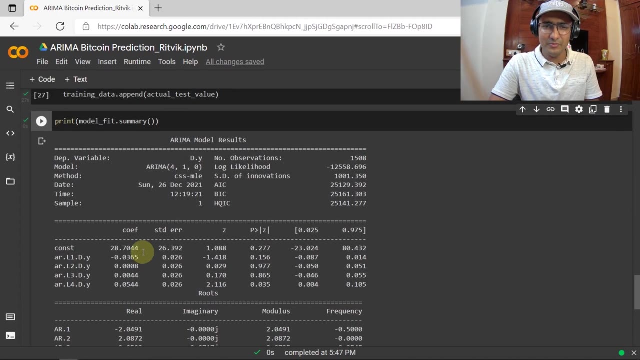 and there are other numbers, such as what is the coefficient of for different parameters, the standard deviation value, the p value, etc. and these are ar1, ar2, ar3, ar4 models, etc. so these are the numbers that will give the in-depth analysis of this model. i'm not going into these details because this video is. 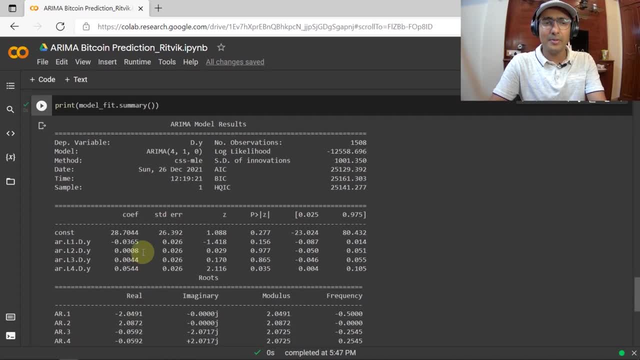 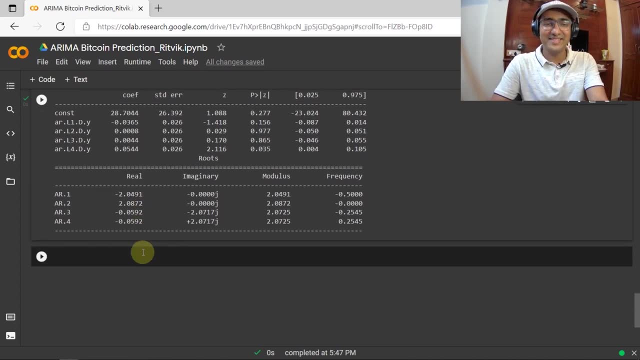 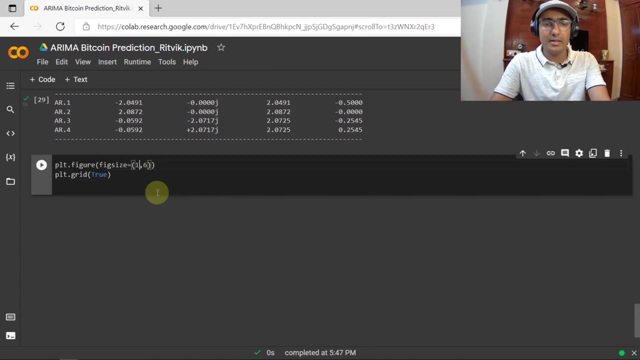 specifically made for the beginners, so i'm just like focusing on the implementation of arima model, right? so now let's visualize the data through a graph, right? that would be amazing. so let me just copy and paste these a couple of lines from here to here, and let's make it 15 and 9. i want a bigger graph this time. so for this, the date. 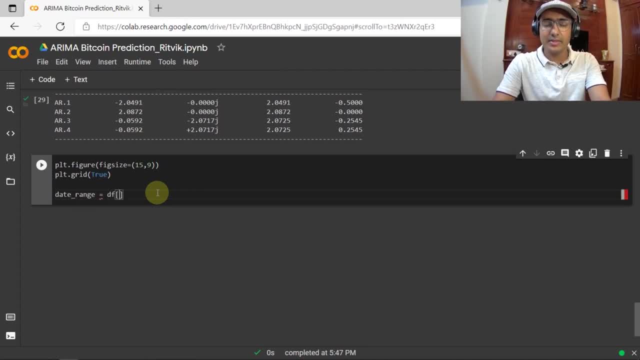 range would be. i'm just interested to see the testing results right. so df and then two row till the end, which is actually representing the testing data, and then index. so the date range is, of course, in the index. perfect now plt dot plot. i will start with date range. 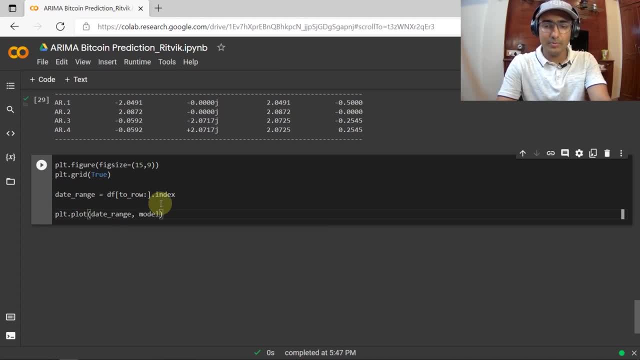 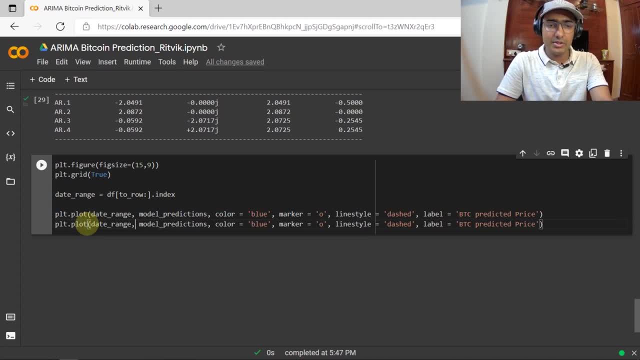 btc predicted price. similarly, plt dot plot date range. and then this one should be testing data color. let's make it red and let me delete all these things here. the label would be btc actual price. i won't take much time, so i put title: is equal to bitcoin. 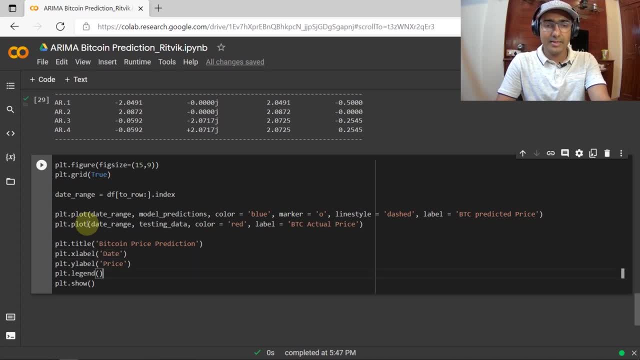 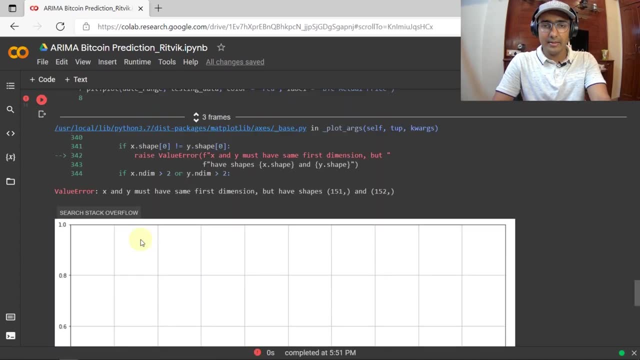 uh price prediction: x label to be date, y label to be price and legend uh will show the legend as well. in the end, plt dot show. let's see the final result. so i'm getting an error here and the error states that x and y must have the first dimension and 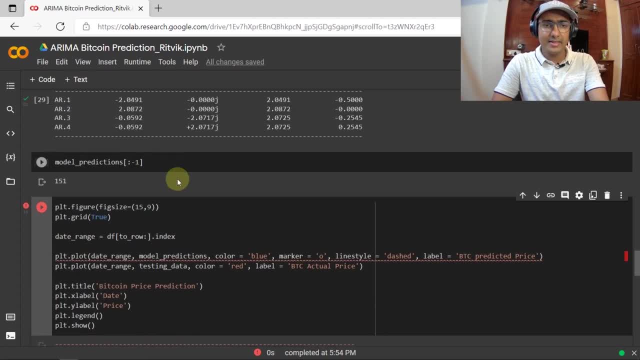 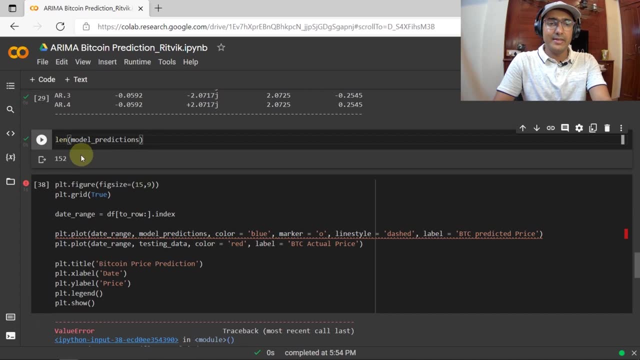 the shapes are 151 and 152. so i just checked it here. uh, if we see model prediction and i'll just write len, the value is 152 and if i write testing data here, the length is 151.. now, why is this? the difference of one is: i think it's because of the decimal. we turned, uh, that float into an. 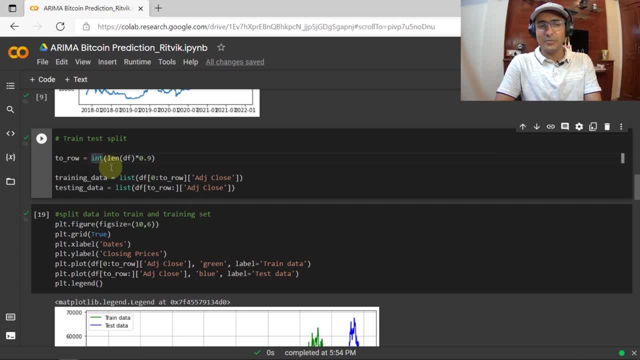 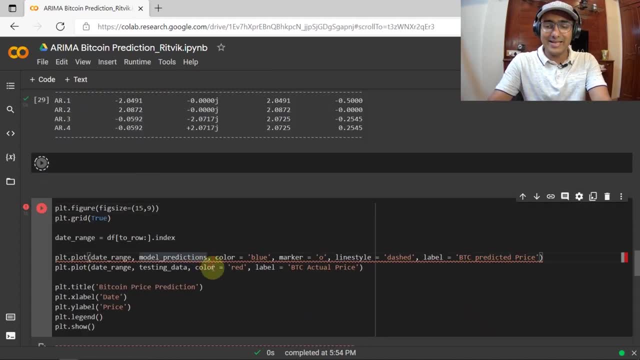 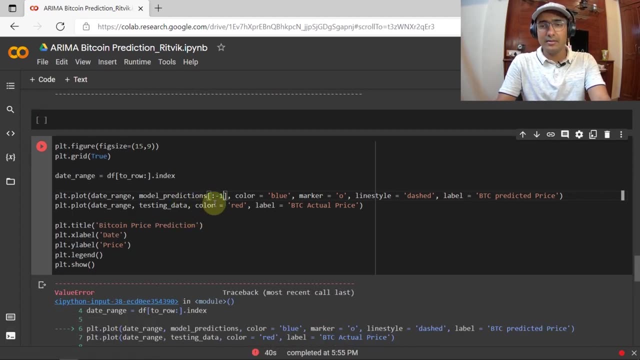 integer, if you remember. uh here, right. so just because of this, uh like, turning it into integer is actually making this error, so i will skip the last one. last prediction, so i'll just go it. go from uh, the first till the second. last one, right, and then let's run this cell. perfect, we have got this. 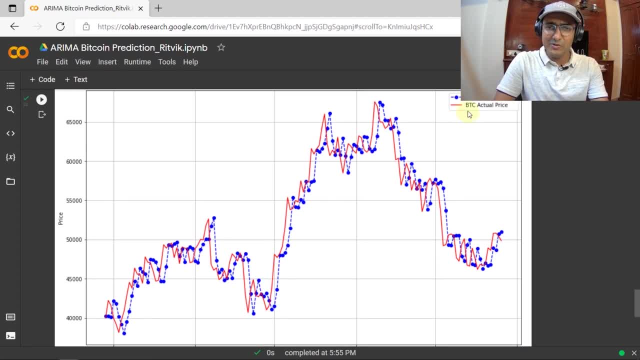 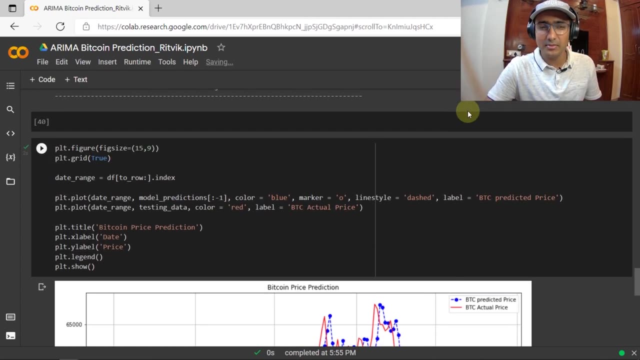 graph and you can see that the red one is the actual bitcoin price and that blue dotted one is the ptc predicted price. you can see that the prediction is a bit lagged. uh, so we'll have to play around with the the numbers here in order to get to somewhat better. 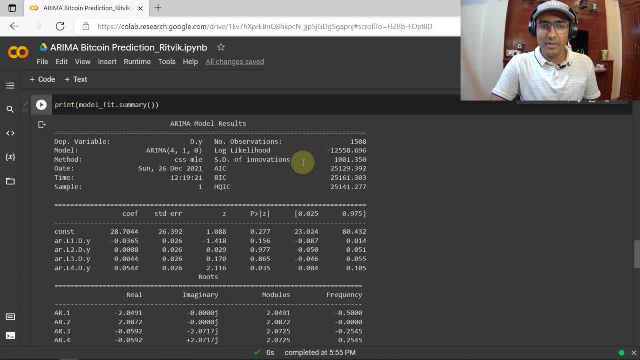 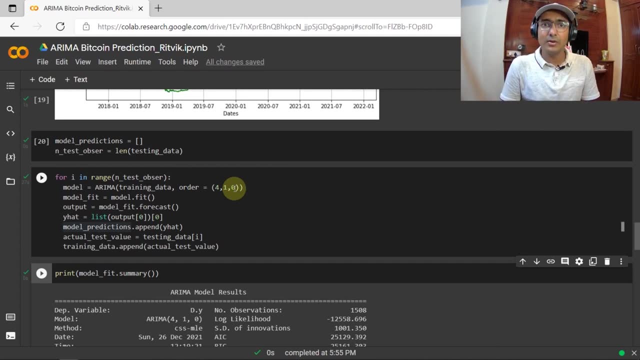 prediction. uh, there's one more thing, guys. if you remember, i just took some numbers such as four, one and zero here in order to represent pd and q. there's another thing called auto arima model, which actually uh does iterations, uh does different simulations for different numbers of p, q and d, and it gives us the best numbers, uh, which should be used as p, d and q. 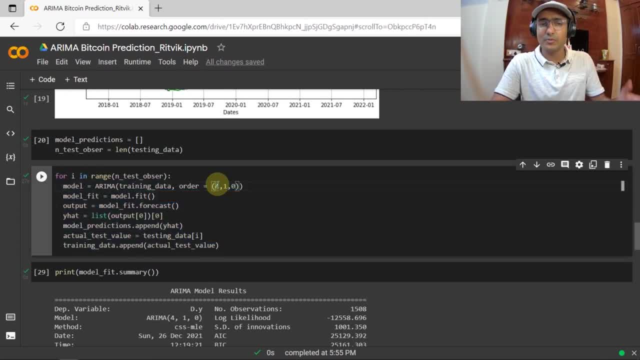 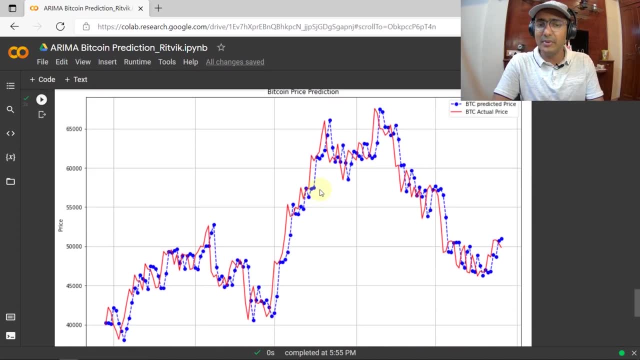 i will try to cover that in future videos. this is just like i just took four one and zero here just to like write this basic arima model. you can see that this model is a bit lagging with the actual bitcoin prices, but it's a very good representation of how we can use this. 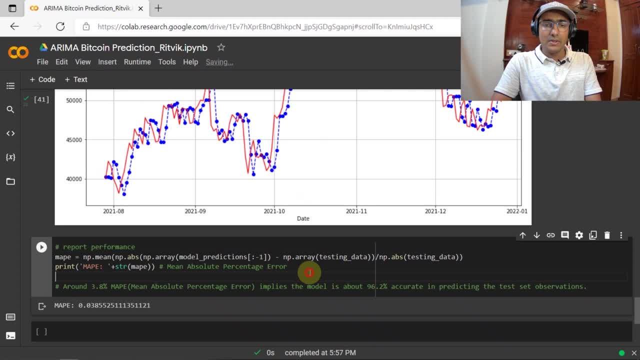 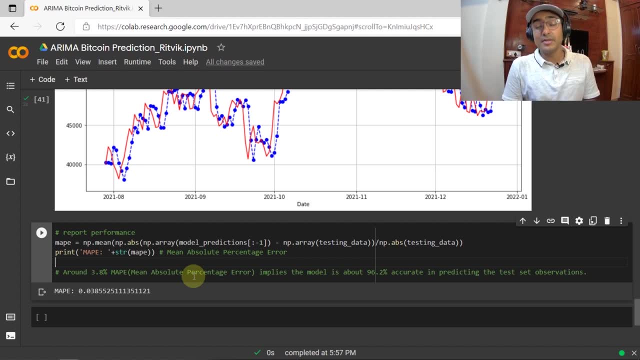 machine learning model to predict some prices right here. uh, i wrote the formula of mape which represents, uh mean absolute percentage error, and the formula is basically: we calculate, uh, we subtract this mean prediction value with the actual value and we divide it with the absolute value of the actual value to calculate the. 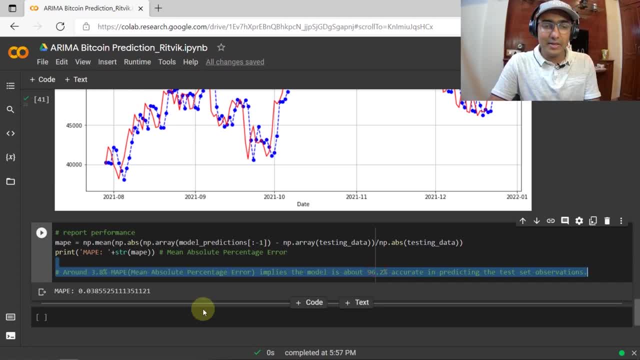 the mape value. in this model we got mape value of around 3.8 percent and it says that around 3.8 percent mape implies the model is about 9%- 6.2 percent accurate in predicting the test set observation. it's a very good 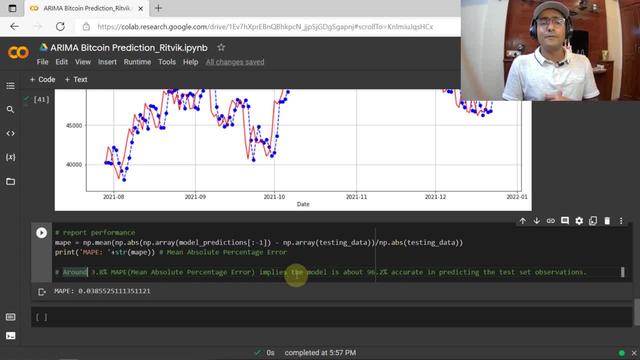 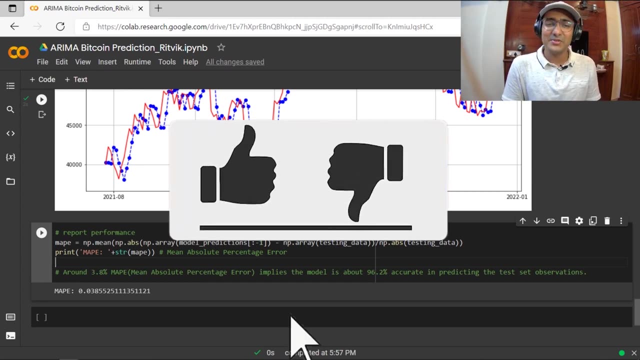 parameter to check the viability of the model. and there are other things which can be used, such as mac, which is mean squared error, root mean squared error, mean absolute error, etc. if you're still watching this video, i deserve one like, at least one like guys. so just like this video and also, uh, subscribe to the channel and commented uh, your opinion, like how. 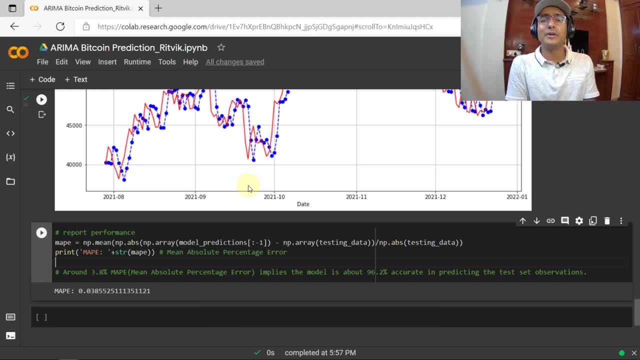 do you like arima model? if you remember, i covered deep learning, lstm and facebook profit in the past, so you can write the comparison of all these three models. i would be really happy to uh, to shout, shout out your name in the next video if you give a very good comparison. 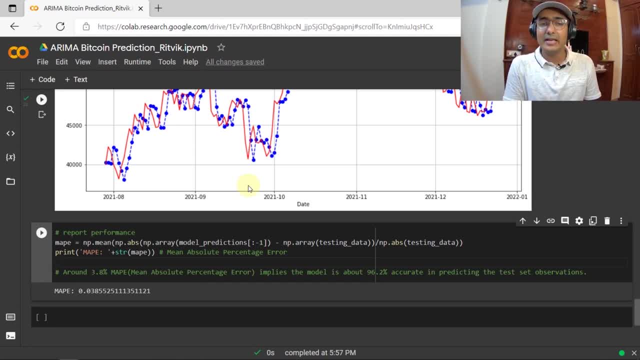 also before before, before getting to know about how to get a free access of my google drive, uh, i just want to introduce my patreon page to you guys. uh, so, yeah, i am active on patreon page and, uh, you can get a very cheap subscription. actually, it's not very expensive, you can see that. 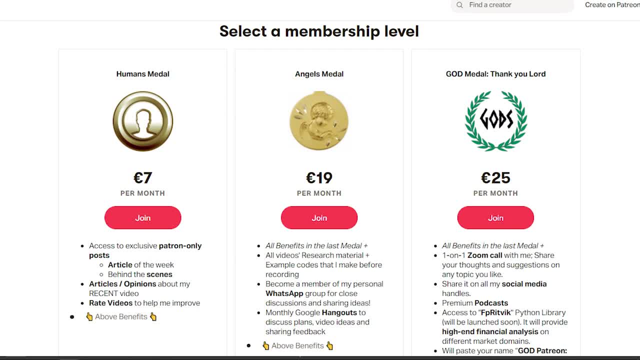 so you can get it over there. there are three different levels over there, which is, uh, humans, angels and gods, and right now i have around seven patreon members. i am very much expecting to grow it further and i recently hired two interns to help me out with this service, and i would be 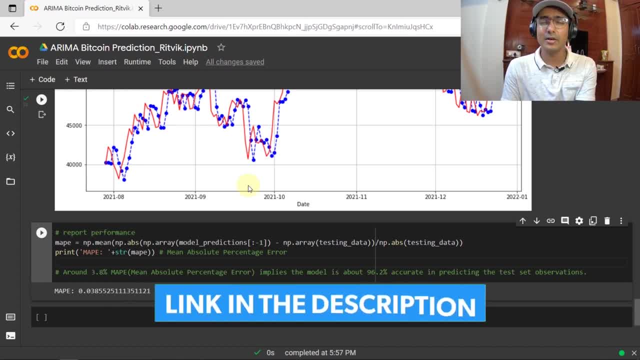 really happy to see you guys over there as well, and this is how you will be supporting my channel as well. now coming back to the google drive, how can you get a free access to your google drive? you just need to subscribe to my youtube channel and click on this button, which is access to my